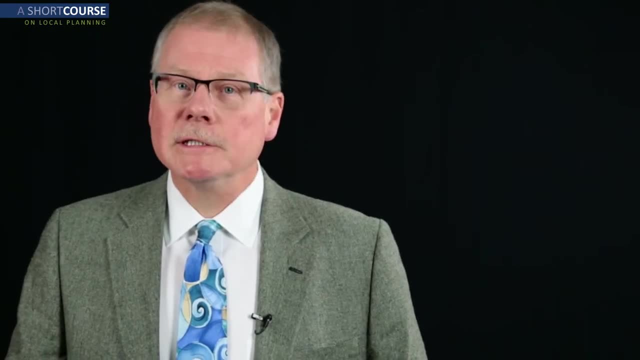 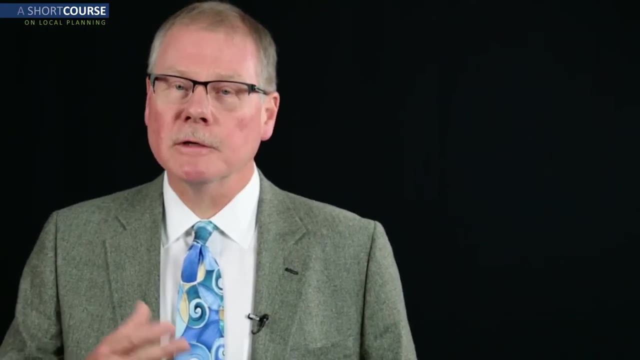 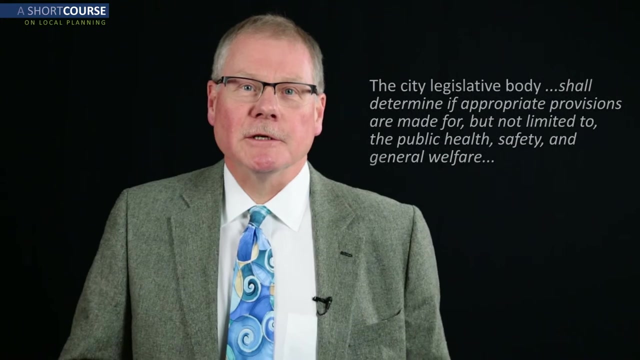 or to an appeal to court if necessary. The hearing examiners and planning commissions that review the plat applications are authorized by statute to require conformance with regulations and there's a long laundry list in the statute about those kinds of regulations. Some conditions are tied to the public health, safety and welfare, which is an important 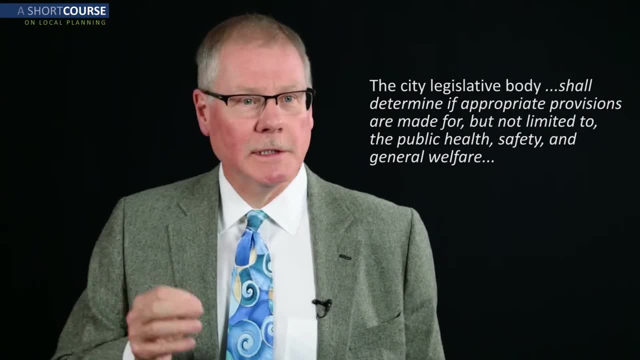 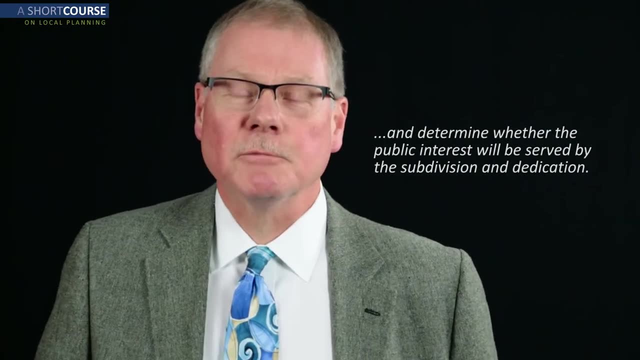 criteria in the law and some of the specific requirements relate to schools and school district, roads, streets, sidewalks for children so that they can get to school, and the public health, safety and welfare and other conditions that support infrastructure needs relative to the public health, safety and welfare. 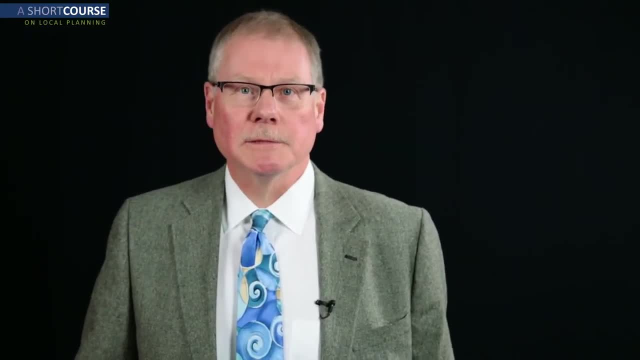 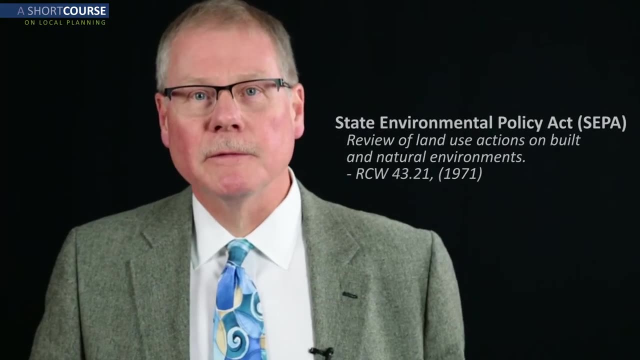 In the early 1970s, by citizen initiative, there were two important laws passed that affect land use planning and zoning. One of them was the State Environmental Policy Act, known as SEPA. SEPA was adopted from the National Environmental Policy Act and 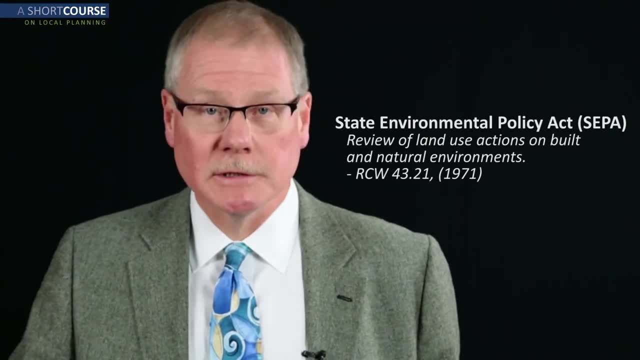 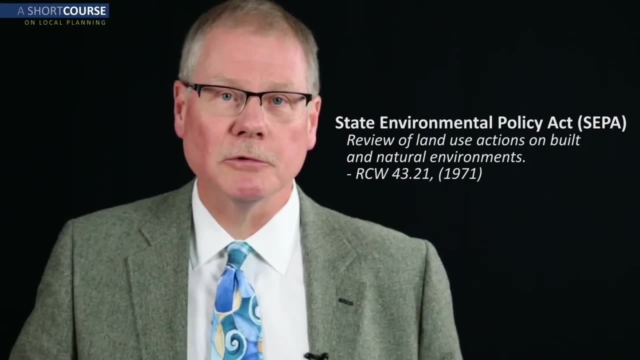 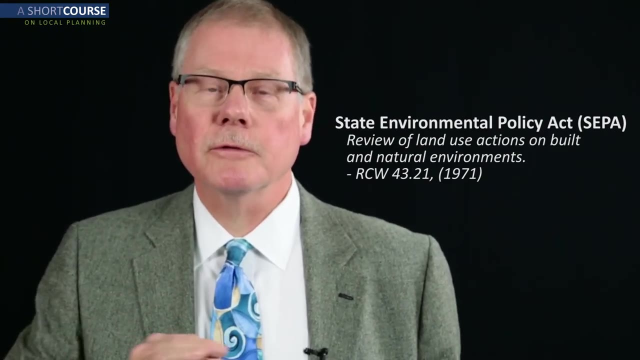 essentially provides a mechanism for decision makers like planning commissions, hearing examiners and city councils to have full information in front of them before they make a decision as to whether or not to approve a development. SEPA is an extensive procedural statute that requires a number of steps as you go through. 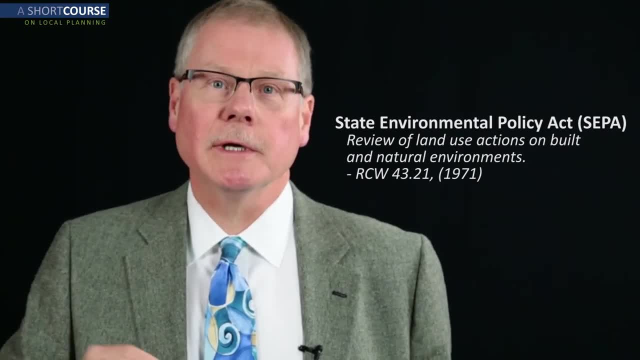 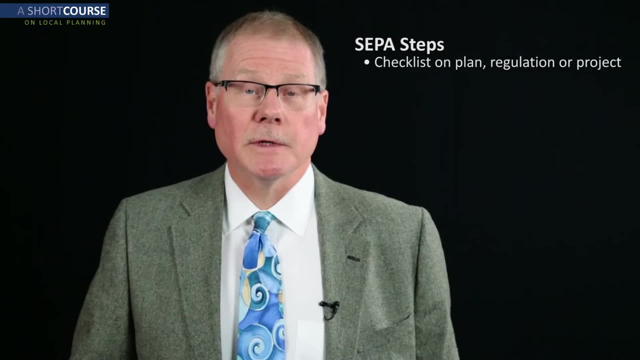 the analysis that it requires, and applies to both the built and the natural environment. Some of the procedural requirements are an initial checklist that comes in with an application, followed by what's called a threshold determination, which could be a determination of non-significance. 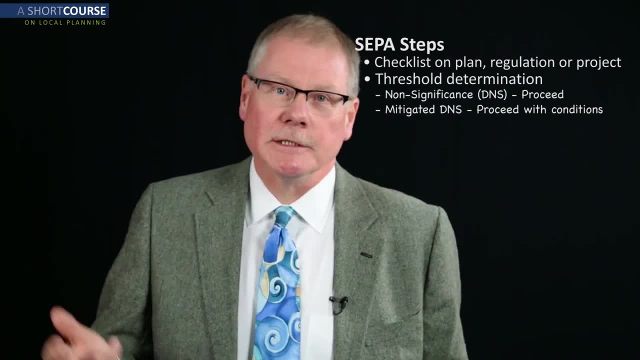 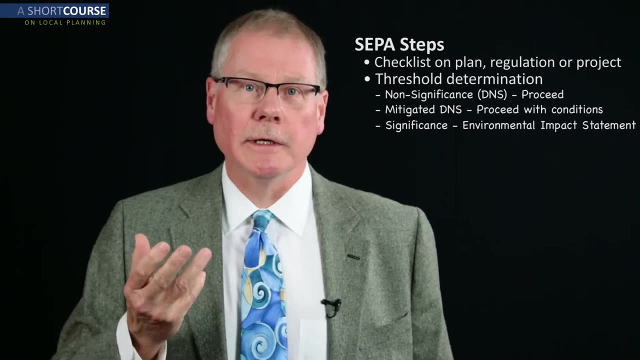 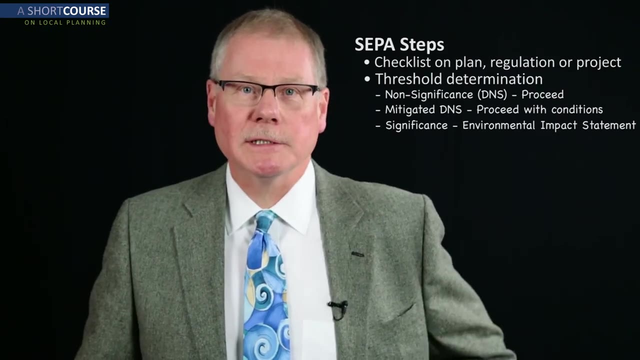 a mitigated determination of non-significance or a determination of significance, and the latter is tied with the environmental policy environmental impact statement or EIS process. When an EIS is required, the jurisdiction will basically call a timeout and it takes about a year to go through that process in 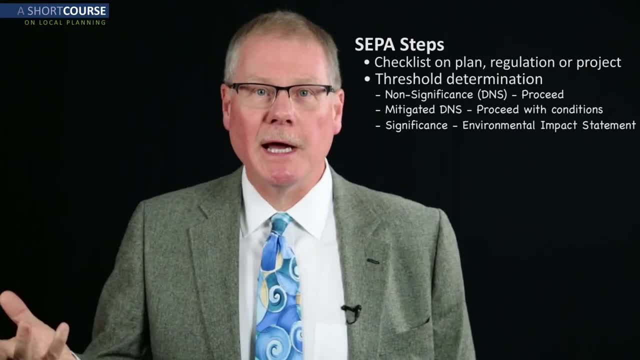 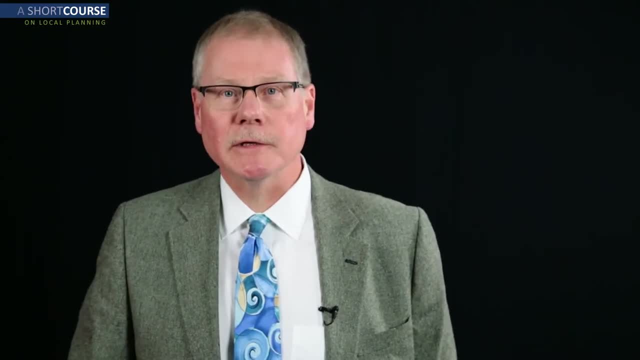 order to create the science and fact-based background to evaluate the project for which it's been prepared. If an ordinary threshold determination, like a determination of non-significance, is made, the project just flows along. naturally, SEPA is required to be performed at the same. 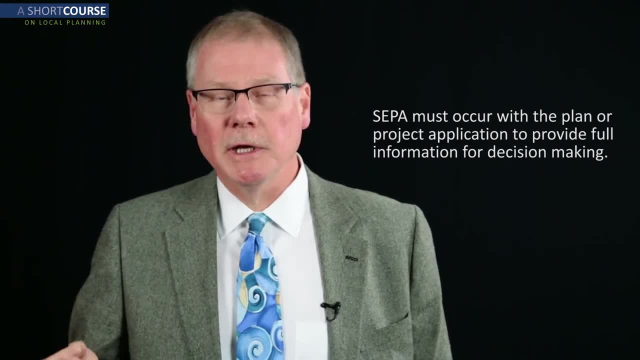 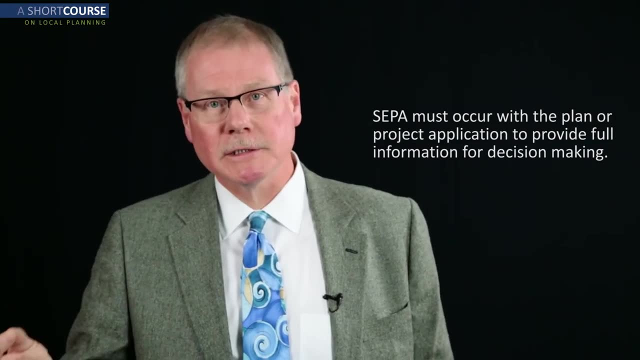 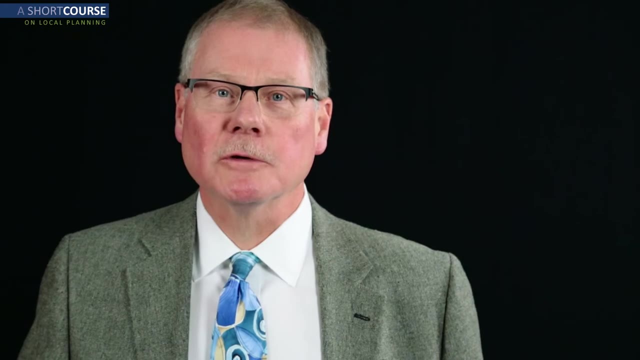 time as the underlying application is presented to the planning commission or hearing examiner, so that all of the information necessary for the decision is available and can be properly considered in determining whether or not the application should be granted. The second major statute adopted in 1971 was the Shorelines Management Act. It was also